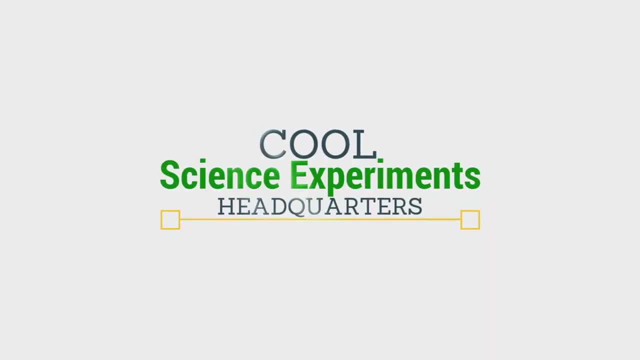 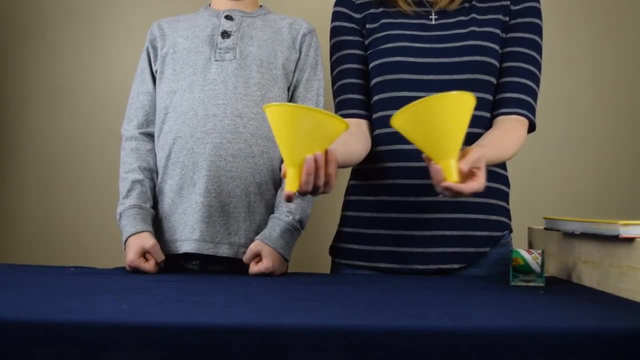 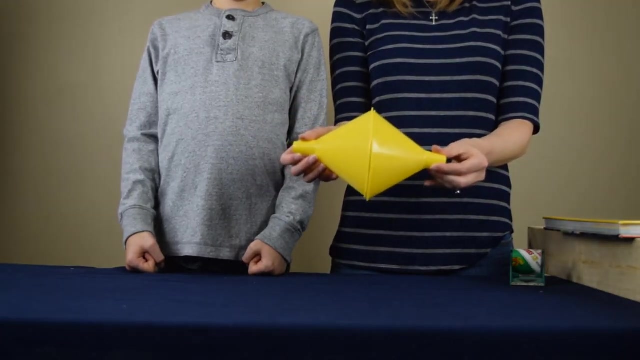 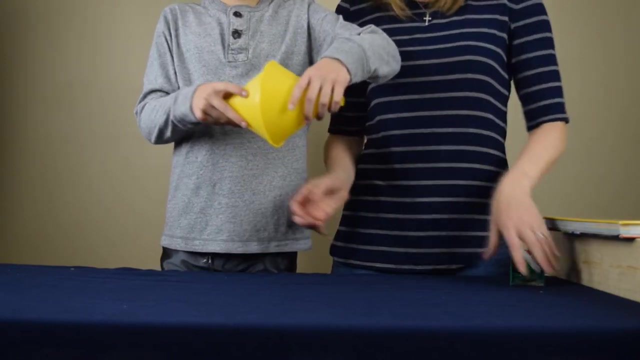 get started, To begin the experiment, you need two funnels that are exactly the same shape and size, And what you're going to do is you're going to put them together at the wide part of the funnel and you're going to secure them with tape, And we're going to put a piece of tape. 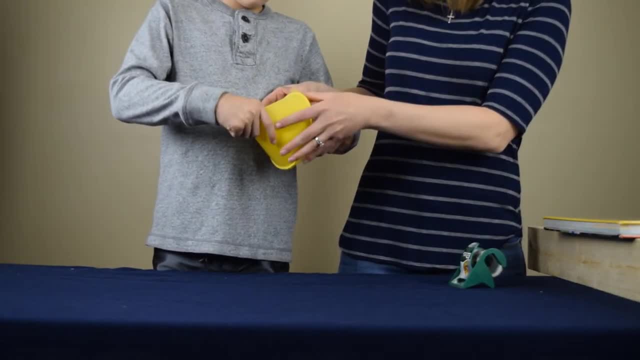 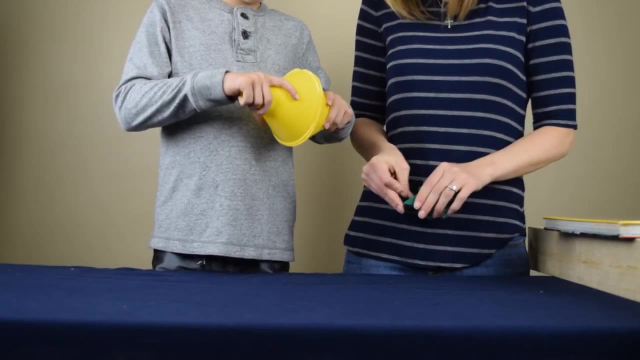 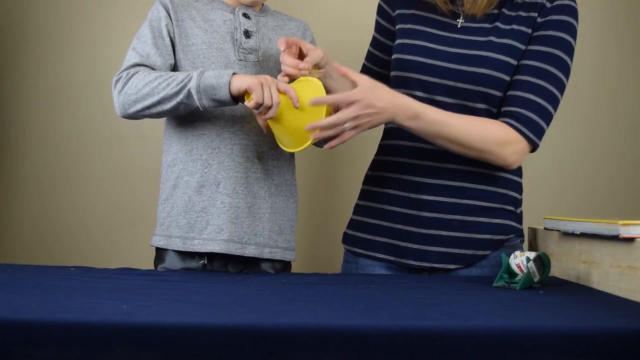 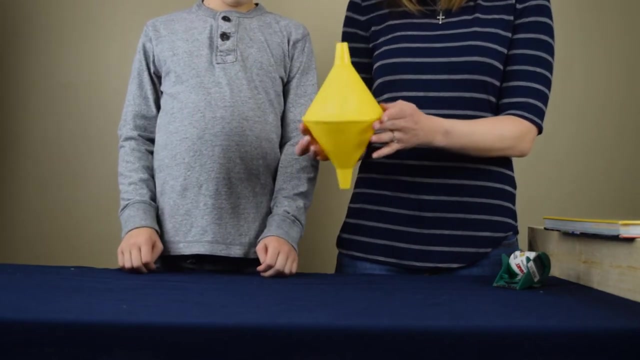 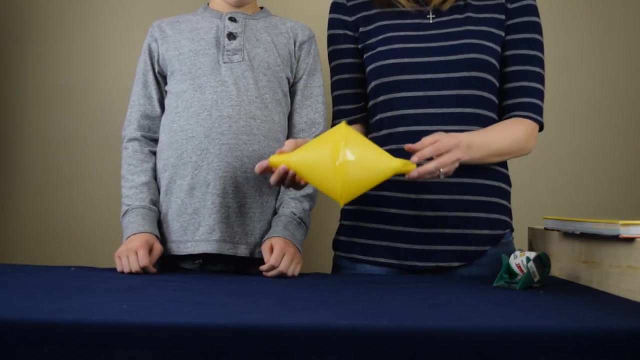 on one side of the funnels, then we're going to turn it around and we're going to put another piece of tape on the other side. So, as you can see, we now have our two funnels that are stuck together with the tape, And 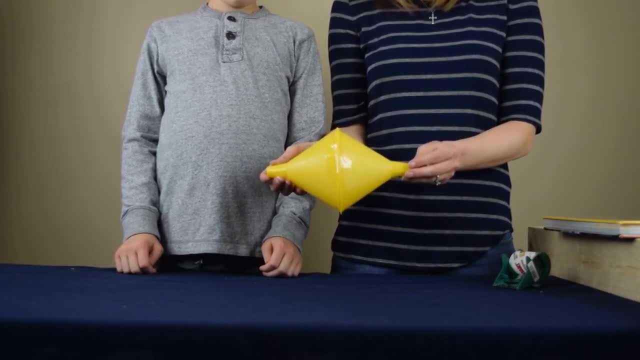 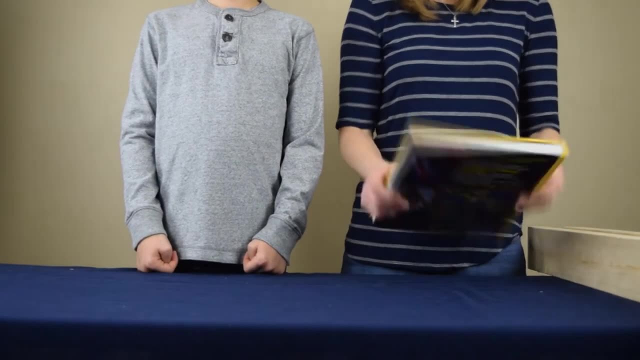 once you have that done, you're ready to move to the next step. So go ahead and set them aside for a moment. To set up the next part of the experiment, you need a large book that is about an inch thick. You're going to place that book on one side of the funnel and you're 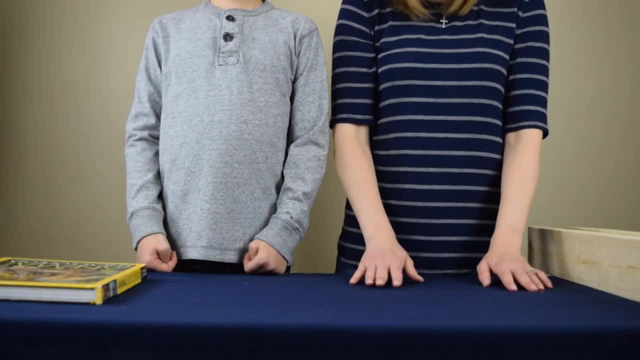 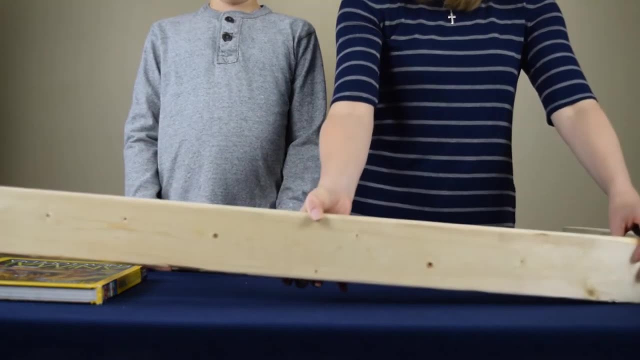 going to put the two wall boards on top of the table. at the bottom of the table and on the floor. You also need two two-by-four boards. What you're going to do is you're going to rest one end of the two by four board on the book and the other end on the table or the. 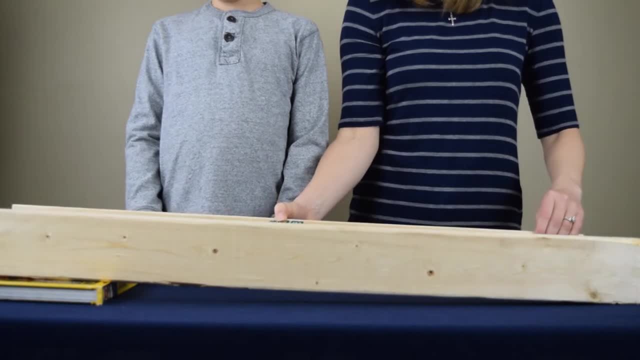 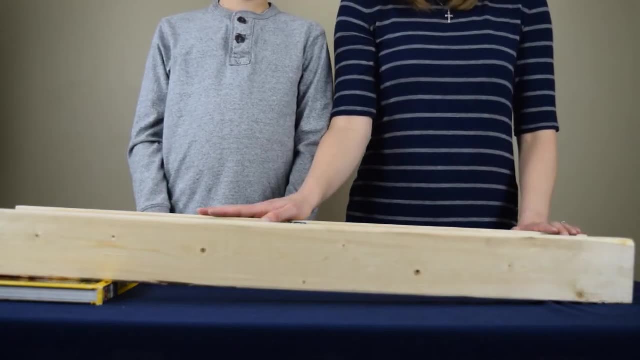 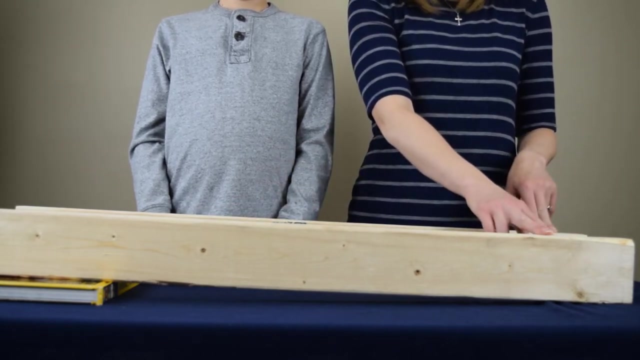 floor. You're going to put both boards side by side, about six inches apart, so they're parallel to one another. So now it's time to adjust how the boards are positioned. Start moving the ends of the boards that are not on the book close together, And what? 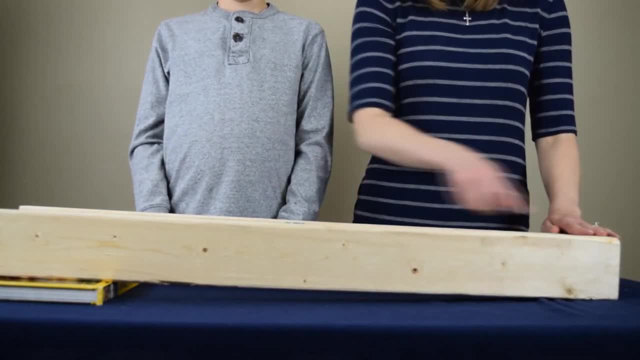 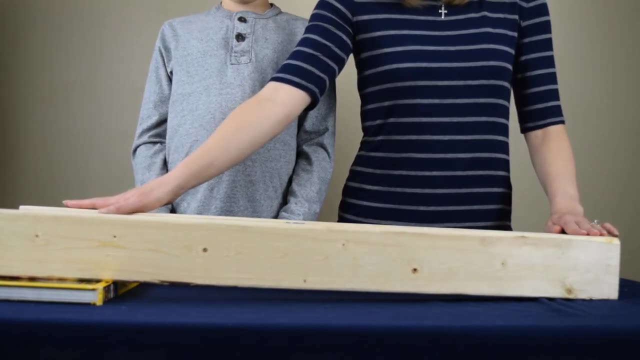 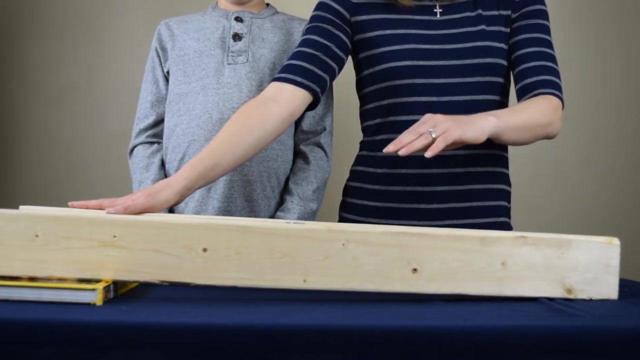 this does is create a V with the board, because this end is close together and this end is far apart. So now I'm going to show you what it looks like from a top view. Now that you're looking at the boards from the top view, you can clearly 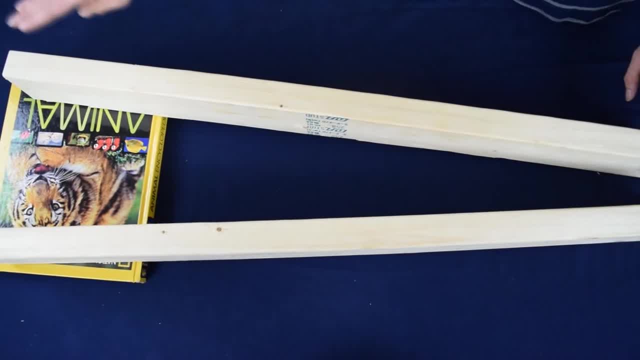 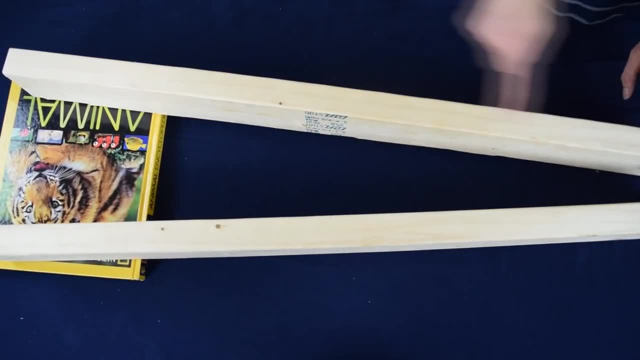 see the V position that we created. The side of the boards that are resting on the book are wider than the side of the boards that are resting on the table and that makes our V shape. It may take a little trial and error to get the